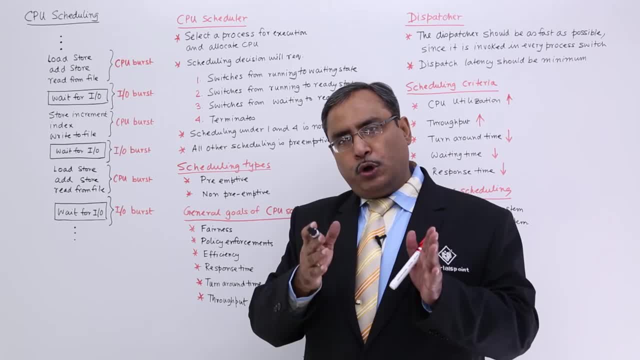 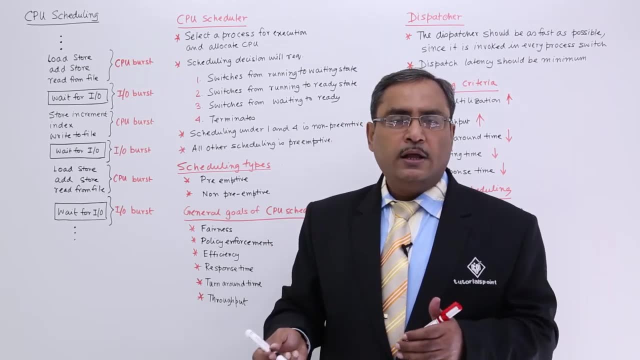 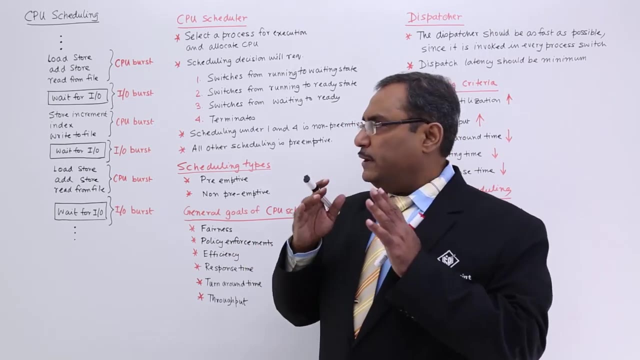 reading some data from some data file, Then whatever it has been produced after doing the calculations, computations, it has to be written onto a certain other target data file. So input output is required. For input output operations it must be getting some data as input from the keyboard. So for 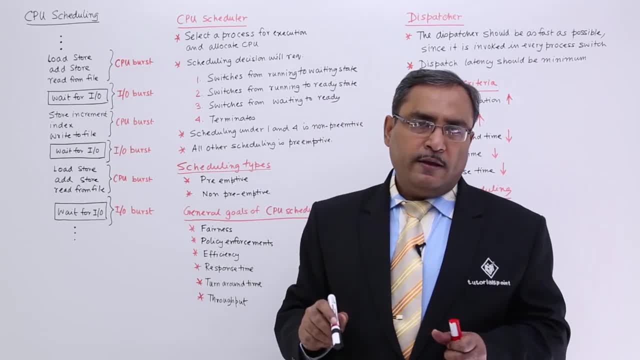 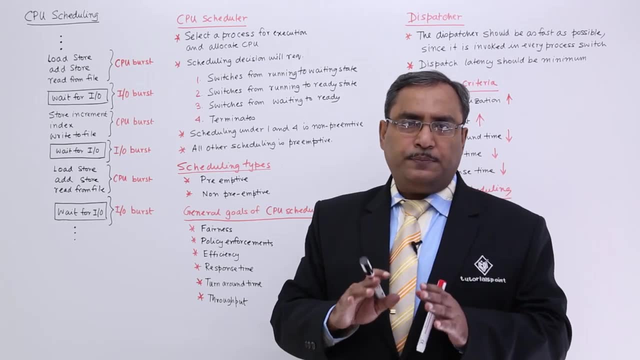 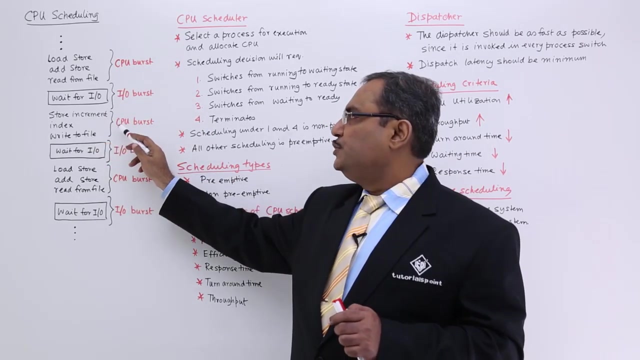 the input-output operation, it will wait for the I O. Frankly speaking, during this period of time the CPU will remain idle. It does not require the CPU access And this is known as the I O burst time, Again for some execution of instructions. CPU burst time, Then wait. 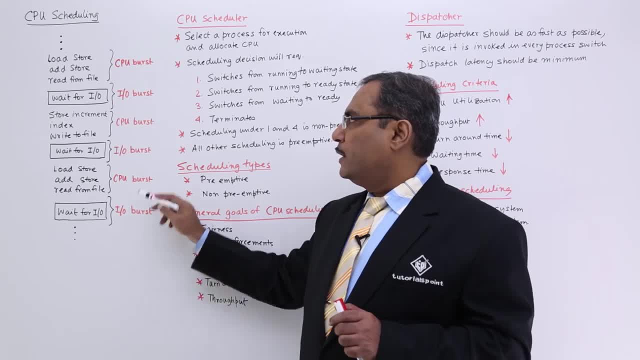 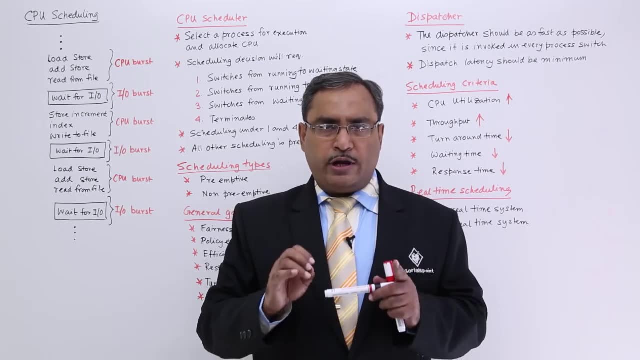 for I O, I O burst, CPU burst, I O burst, And so on. In this way, we are getting the idea that a process during execution does not require the CPU at a stretch. As a result of that, during that period of time when 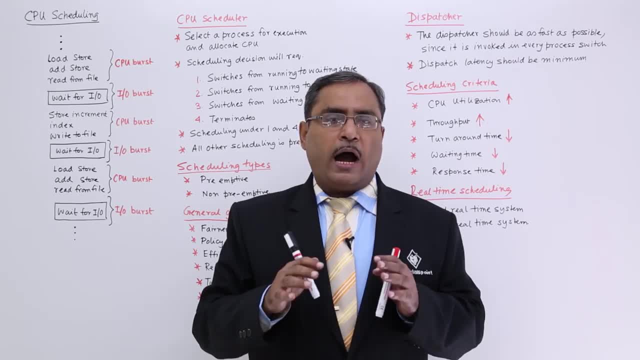 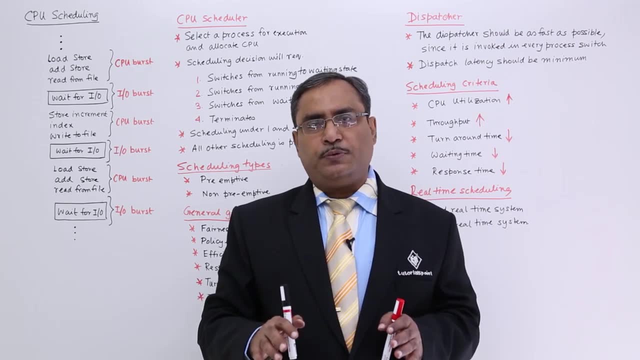 the process is getting busy for some. I O wait or I O operation. and you know that input-output devices are slower devices compared to the speed of the CPU. So all the CPU will have to wait for the input-output operation and that might be a long time. So this is known. 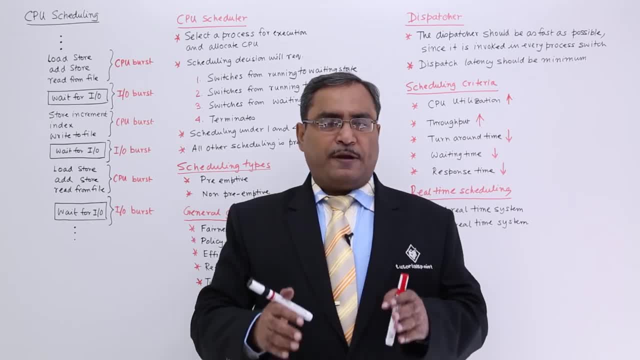 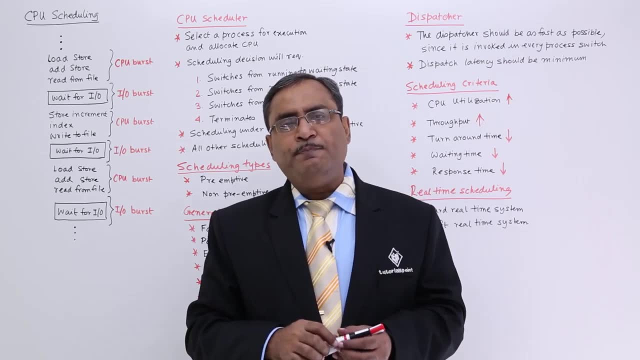 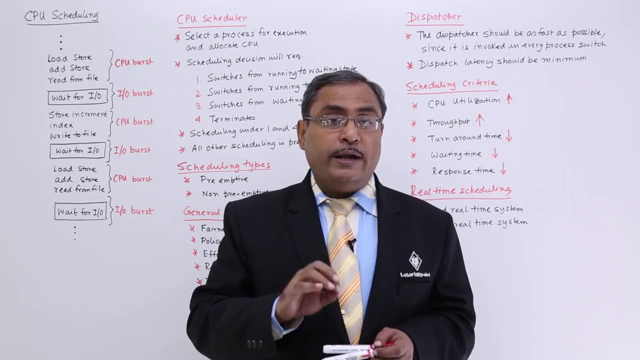 long duration of time. So, during this period of time, if I find that in case of multi-programming environment, wherever multiple processes are existing in the computer's memory, if you find that there are some other process existing in the memory, they are requiring CPU interaction. 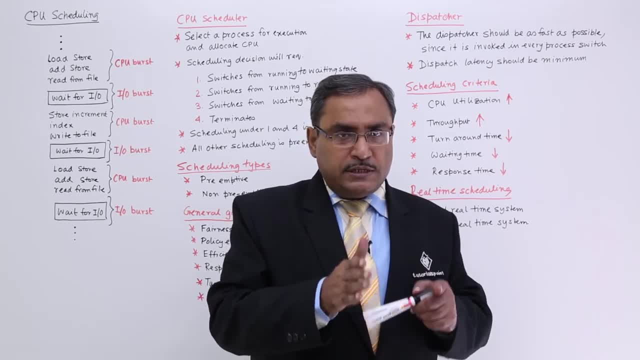 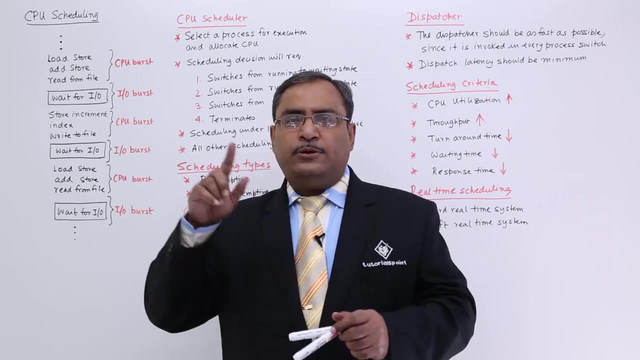 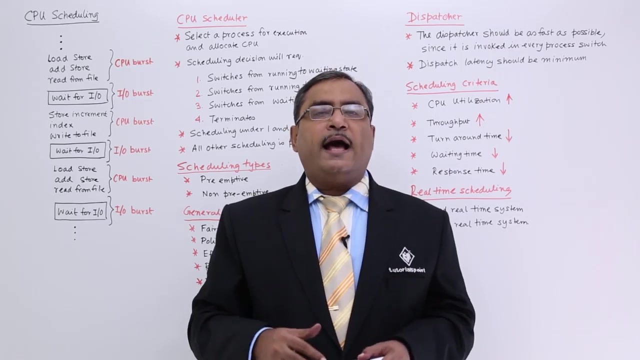 then, during this period of time when the process is busy for the IO operation and leaving the CPU in the idle state, then that particular CPU will be assigned to that particular process which is requiring CPU interaction right now, So that in this way we can enhance the CPU. 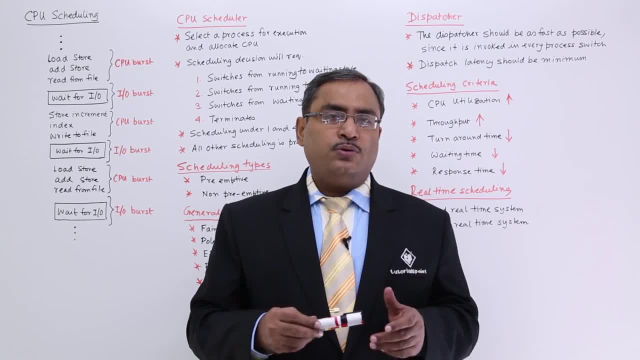 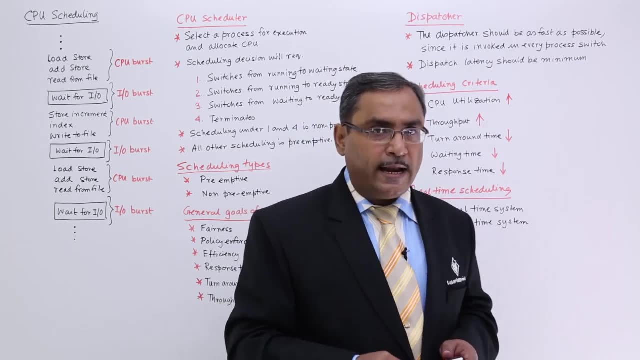 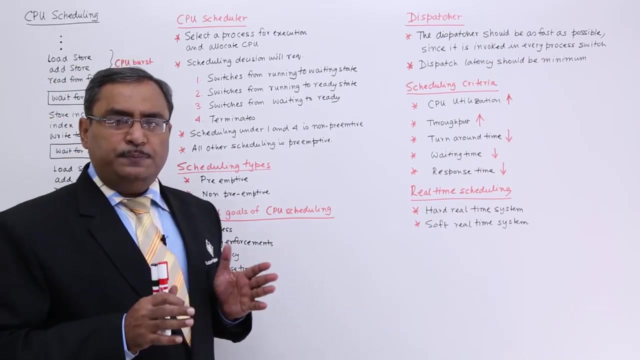 utilization and performance of the system. So this is known as the CPU scheduling and for which this particular subject or the topic has arrived. So now you see the CPU scheduler. What is the CPU scheduler? CPU scheduler is nothing but a software which will decide that CPU is going to get allocated. 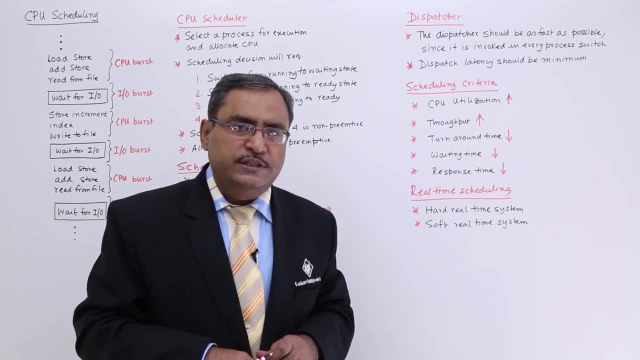 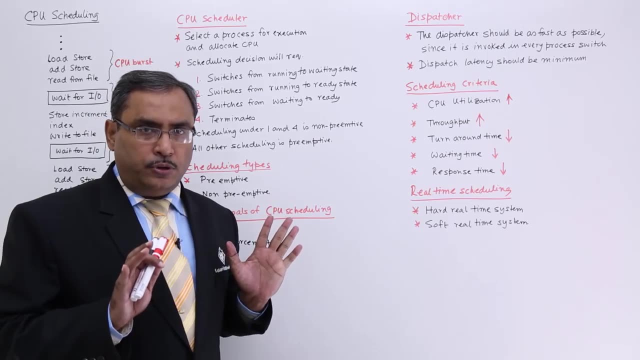 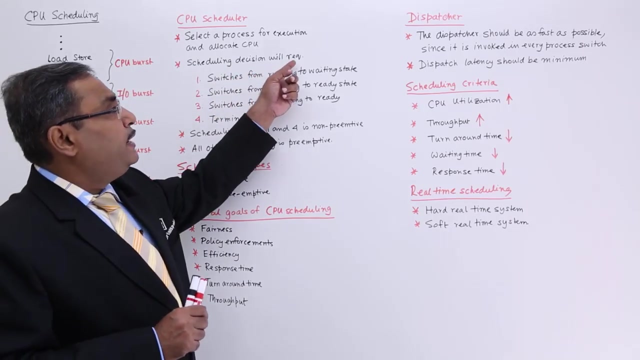 onto which process and that is why it is called CPU scheduler. So CPU scheduler will select a process for execution and allocate the CPU. So that is the purpose of the CPU scheduler. CPU scheduler is a software. Scheduling decision will be required. The scheduling decision will be: 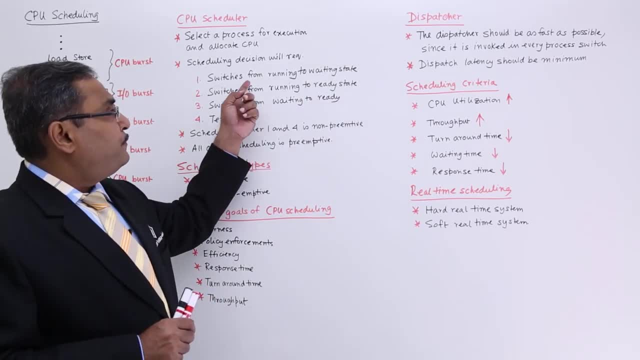 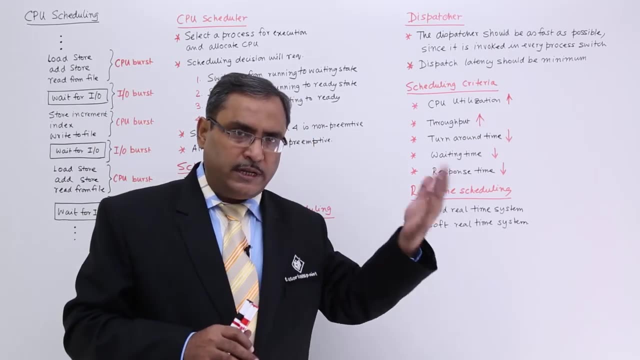 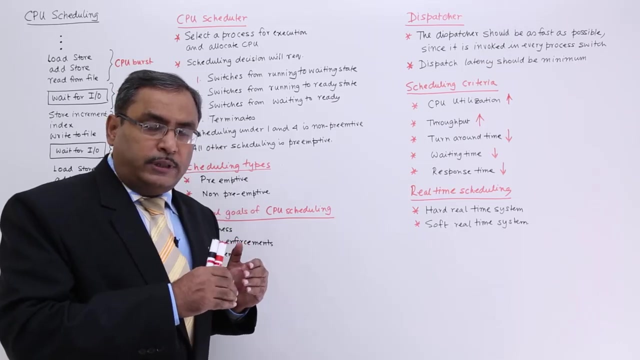 required in the following cases: From the running to the waiting state, Process state transition- We are having a separate video on that. Please watch that one also. So switching from the running state to the waiting state. So when the process is going from the running state to the waiting state, then the CPU scheduling is. 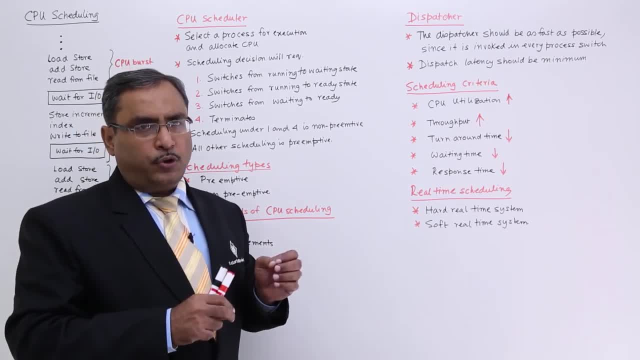 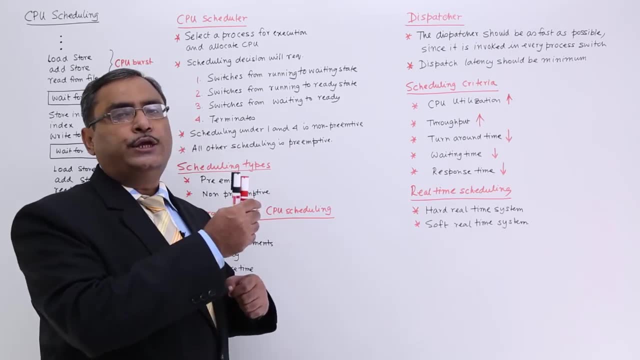 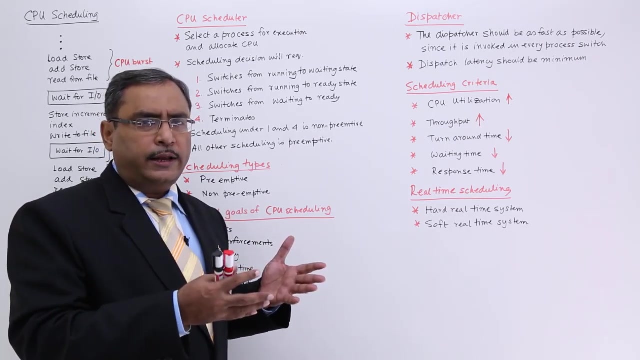 required because I should take out the CPU from the process Switches from the running to the ready state. That means the process was running. now it is going to the ready queue. Why? Due to the expiration of the say time quantum in the round-robin scheduling. So as the 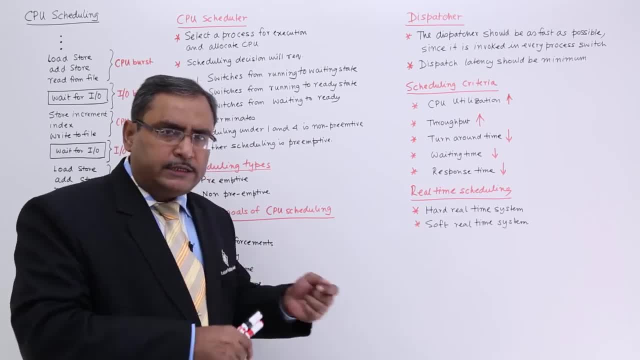 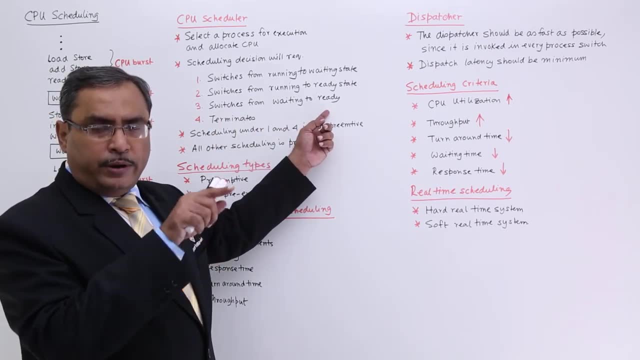 time quantum has expired. so the process from the running state to the ready state. it will be going, Switching from the waiting to ready. so it was in the waiting queue, now it is coming to the ready. In this particular case, the CPU has to be allocated to the respective 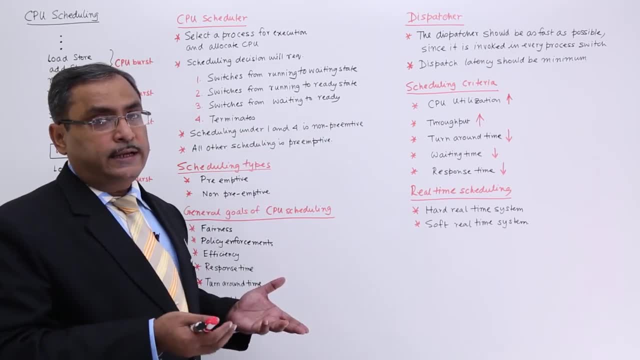 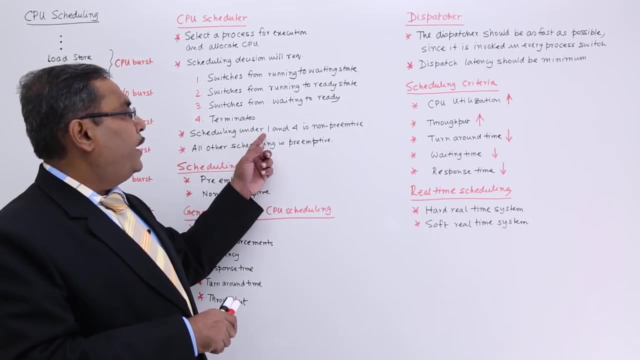 process when the process will terminate. So obviously in that case I should take away the CPU from the process. So here the CPU scheduling is required. Scheduling under point 1 and point 4 is non-preemptive. 1 and 4 is non-preemptive, So we are having two. 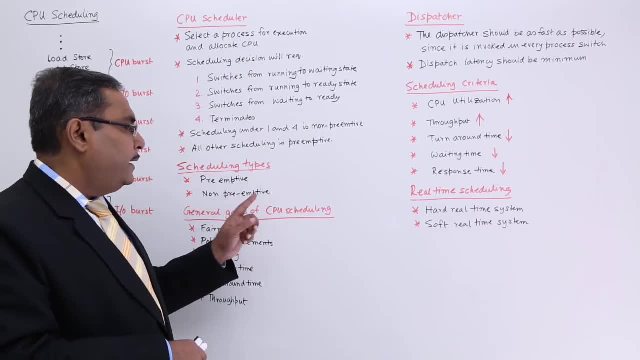 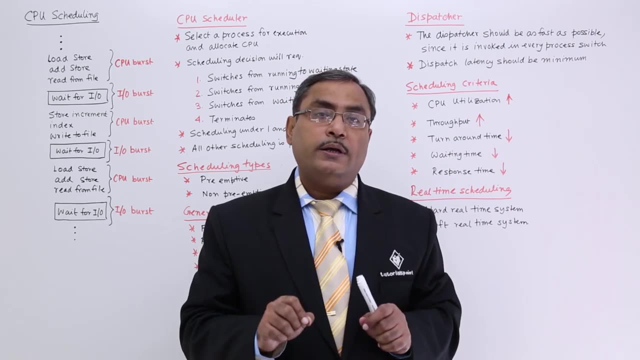 kinds of scheduling: one is a preemptive and the other one is a non-preemptive. In case of preemptive scheduling, if required I can take away the CPU from the process whenever required. But in case of non-preemptive, when the 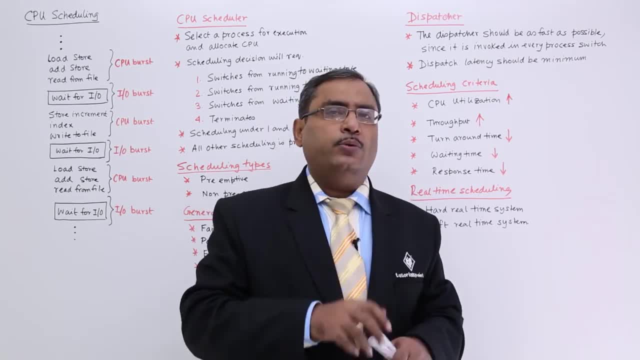 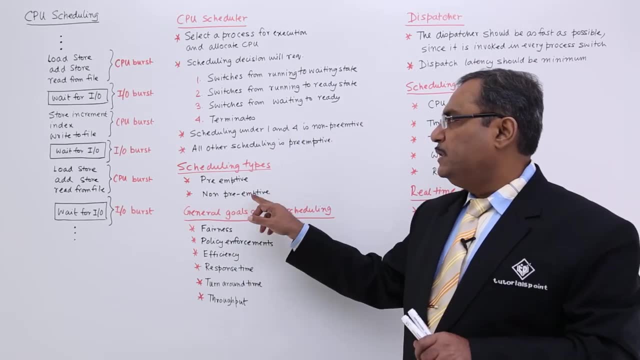 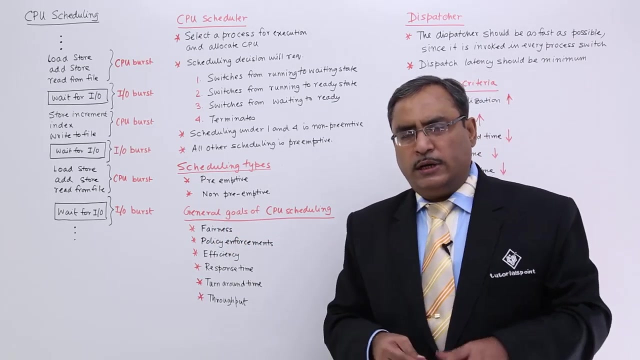 process will relinquish the control over the CPU. then only we can take away the CPU from the process, and this is known as preemptive and non-preemptive scheduling. Now, what are the general goals of the CPU scheduling? One is the fairness. What is the? 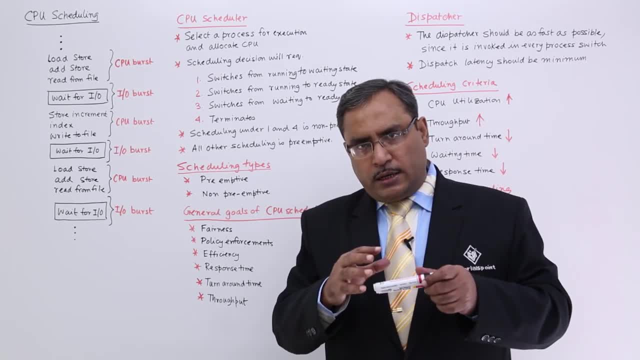 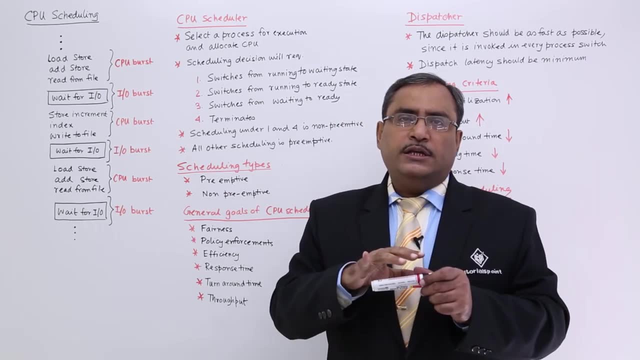 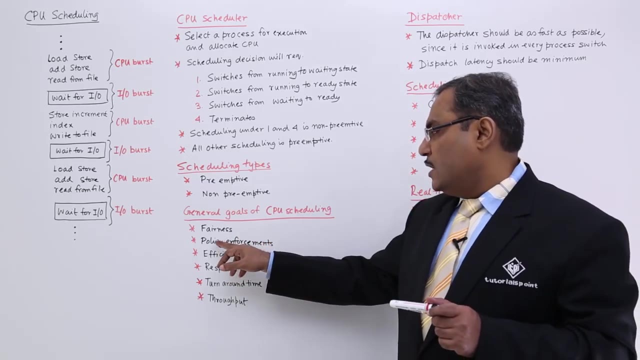 meaning of the term fairness. This CPU scheduling should be done in such a fair way that all the processes competing for the CPU access will get the fair usage of the CPU. So all the processes must have the fair usage of the CPU and that is known as the fairness. 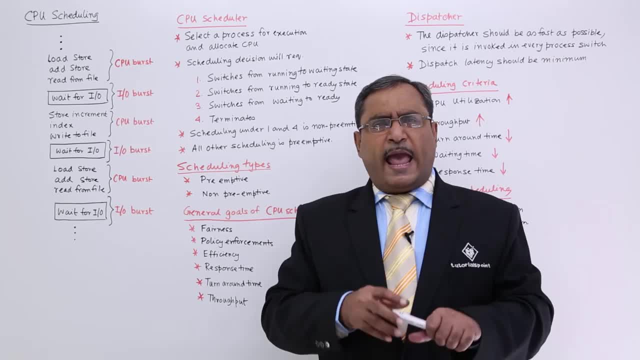 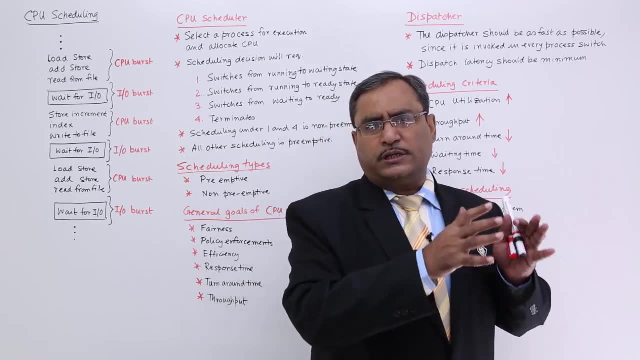 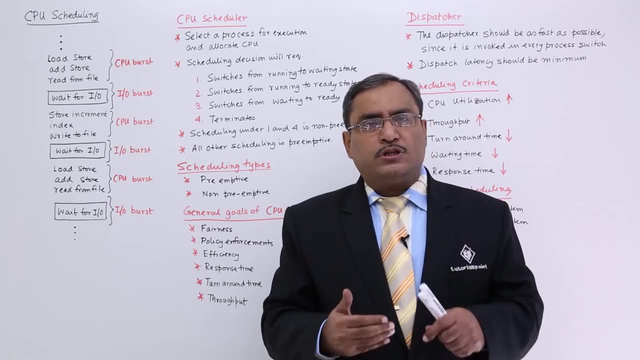 Policy enforcement. let us suppose in a particular system, say, accounting related processes must be coming later than the security related processes, system security related processes. So that is the policy that particular system is having. So whenever processes will be requiring the CPU access, I should give the CPU to that very particular process, which. 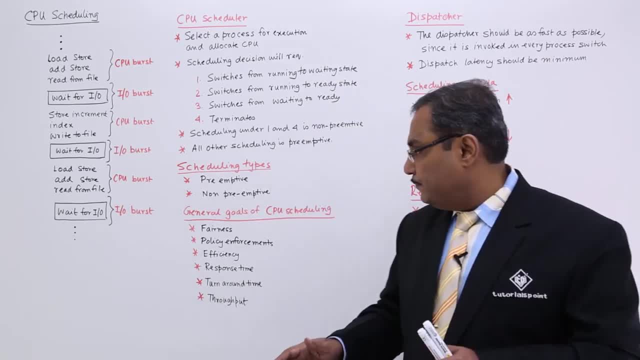 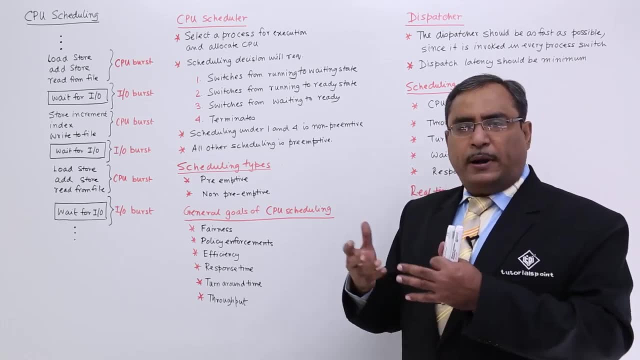 is in accordance with the policy enforced. Now, efficiency, Obviously. I told you earlier that. why should I keep a CPU engaged to a particular process when the process is in the waiting state? So I should take away the CPU from it and allocate the CPU to another. 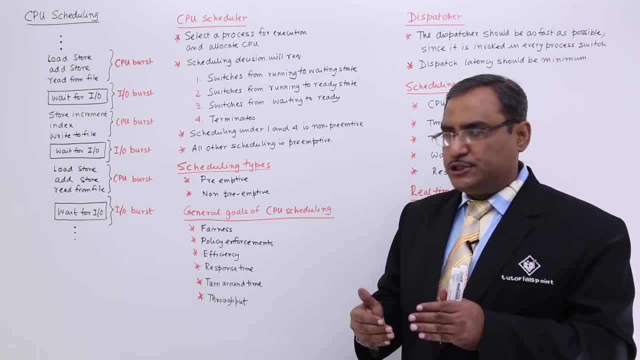 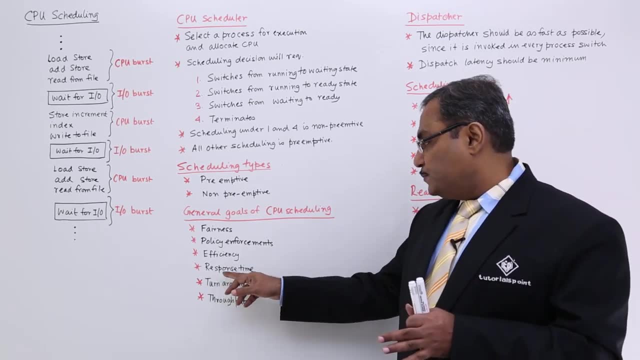 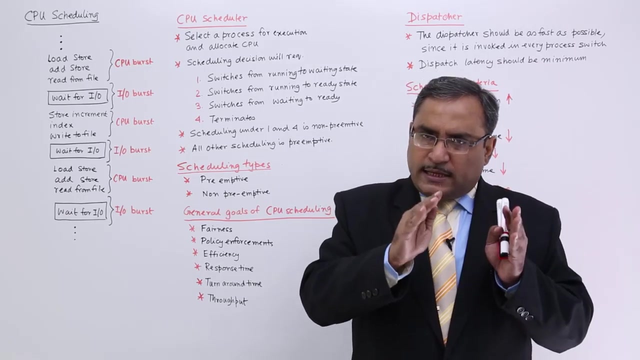 process which is right now requiring the CPU interaction. So that is why efficiency of the system will get enhanced and that is one of the goals. Response time, that means allocation of the process and first response obtained from the system, That means the process has. 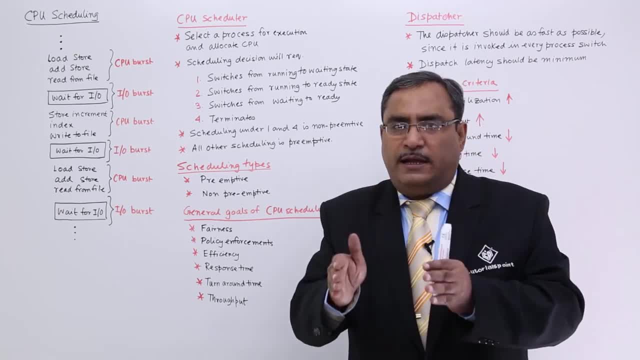 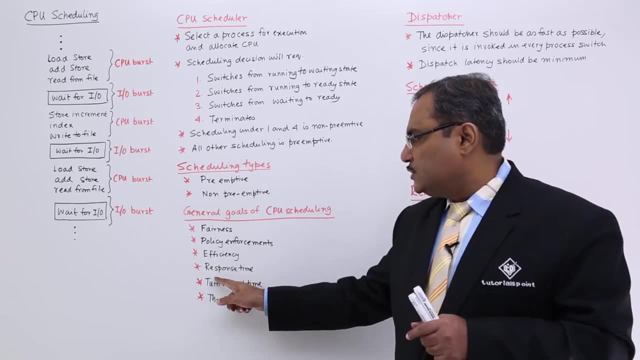 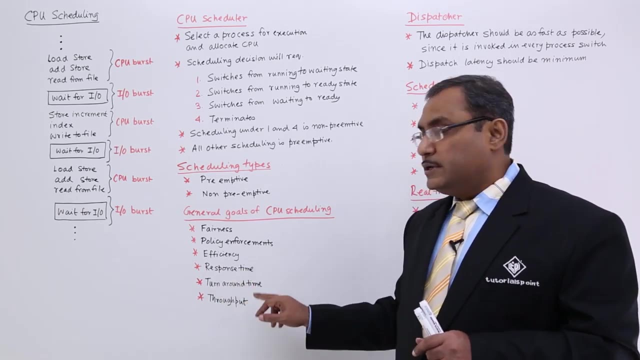 got. the birth is a new process has arrived in the system and the first time the CPU is getting allocated to the process. the time required is known as response time. Obviously, we should decrease, we should try to reduce this particular response time. Turn around time: the process submission and process completion: The time gap is known. 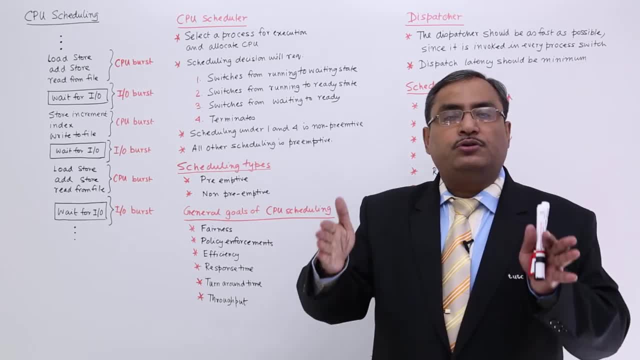 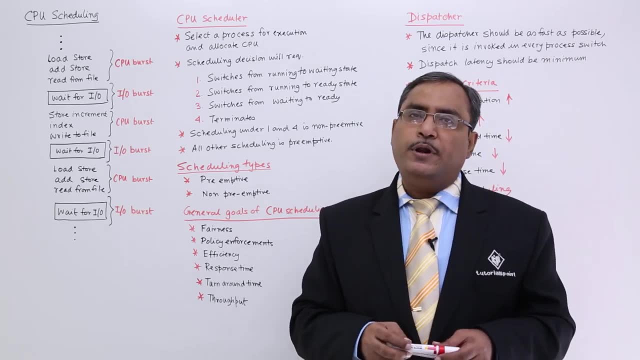 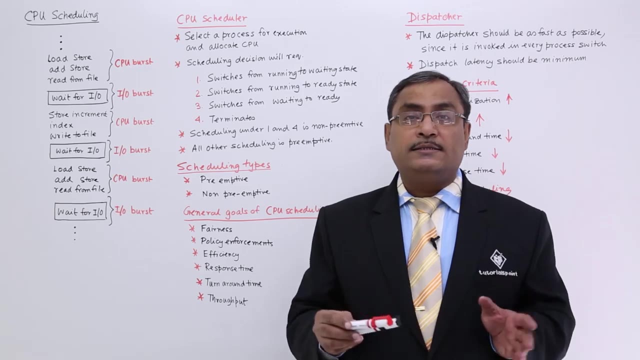 as turn around time time and obviously we should reduce, we should try to minimize this turnaround time and the throughput- throughput means number of processes completed per unit time that is known as throughput. obviously we should have that very scheduling criteria which will enhance and which will ensure the 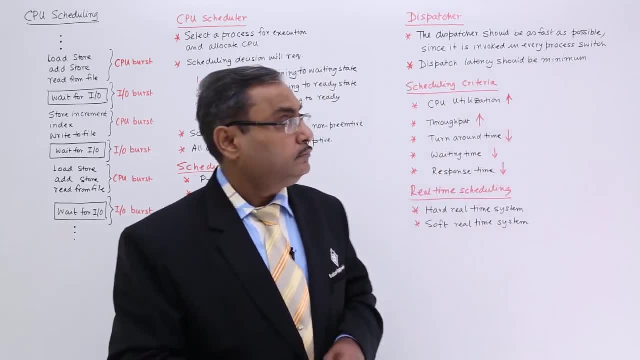 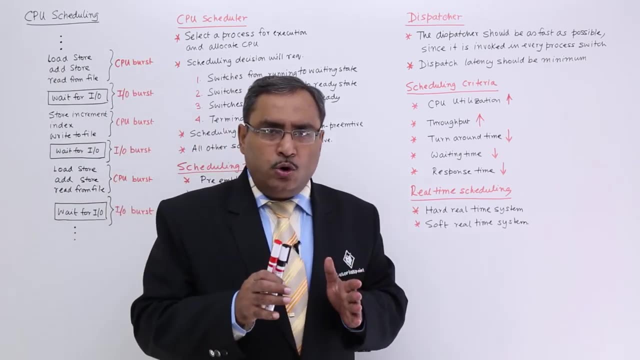 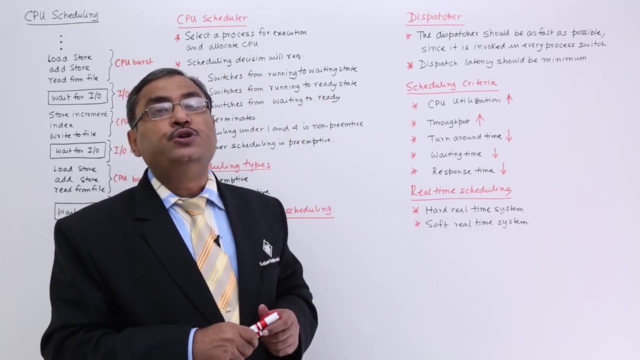 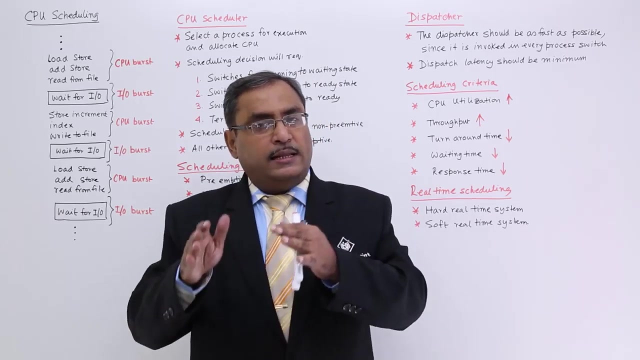 high throughput, maximum throughput in the system. okay, now let me discuss what is a dispatcher. dispatcher is nothing but one software which will allocate the cpu to a certain process, which process which has been decided by the cpu scheduler and this sort of context switching, because you know, whenever we are allocating a cpu to a certain process, then process is going to 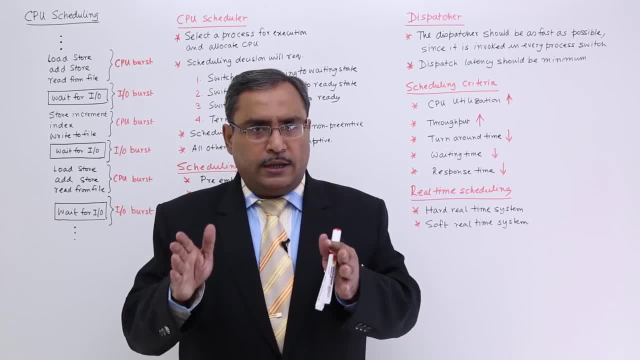 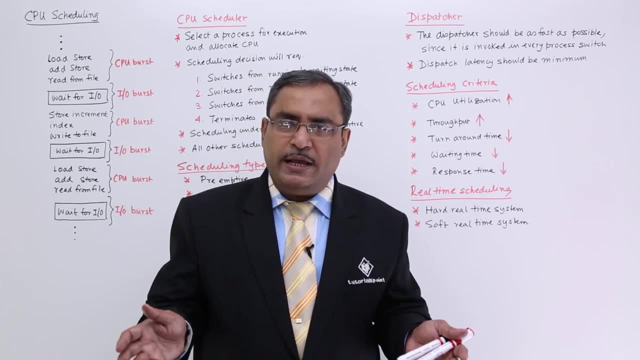 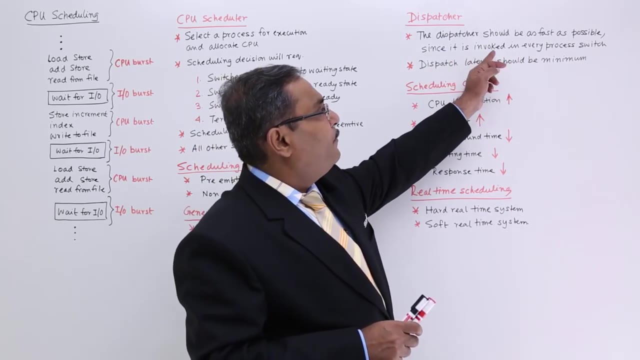 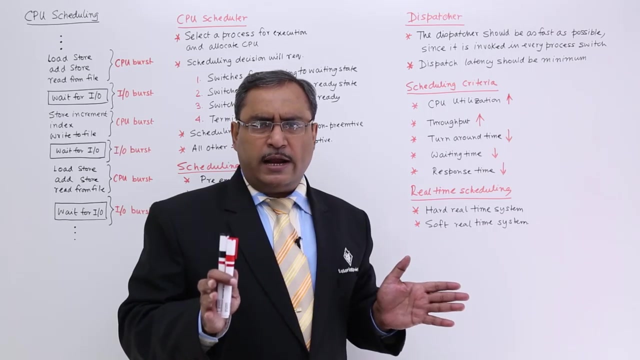 resume or is going to start okay. so this particular context, switching time should be minimum because during this period of time actually cpu is remaining unutilizable. so dispatcher should be as fast as possible, since it is invoked in every process. switch and dispatch latency should be minimum. we know the term latency. latency means delay. 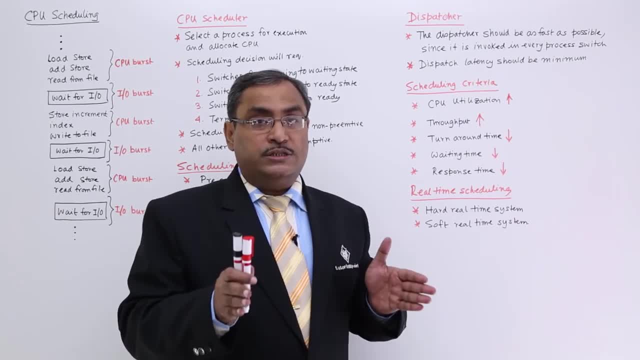 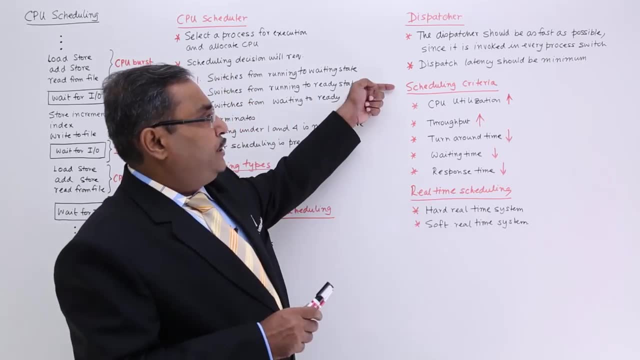 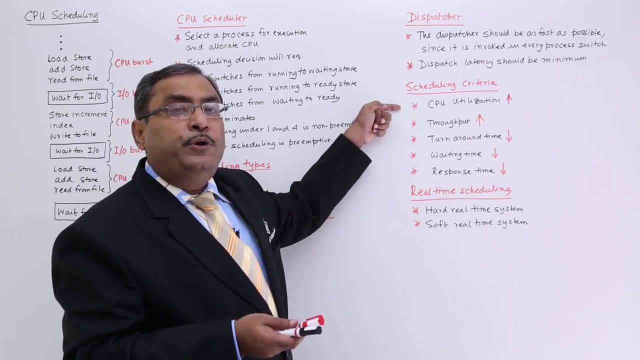 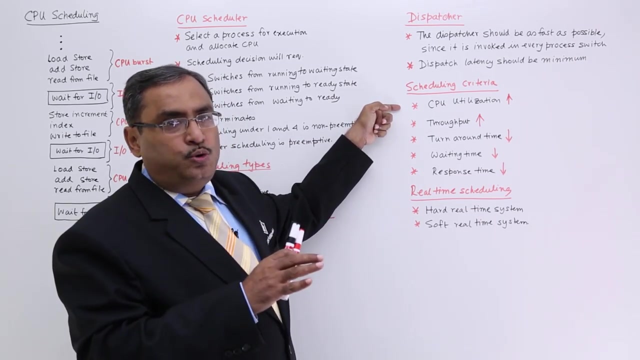 the dispatch latency should be minimum because during this dispatch latency period of time the cpu is sitting idle. scheduling criteria: we should make the cpu utilization highest. that means maximum, rather. i should say cpu utilization means means the percentage of time for which the cpu has been kept busy. tax could be assigned onto the cpu and we know that in case of heavily busy system also. 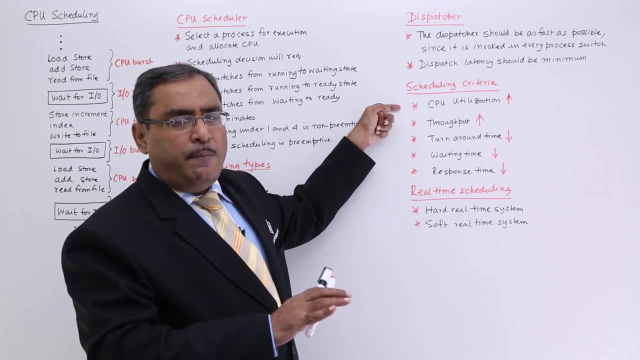 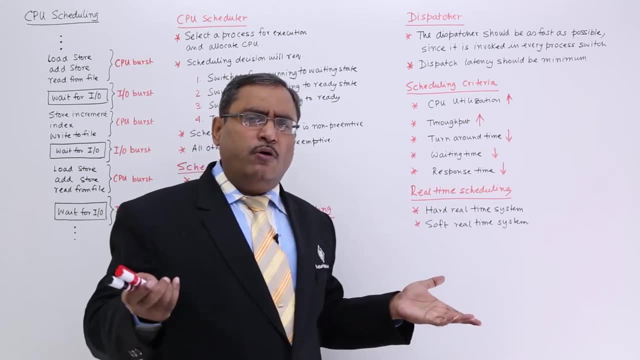 the cpu utilization is very difficult to cross 90 percent because you cannot find a process which is requiring cpu introduction for a long period of time. so always we go for the cpu scheduling and whenever the context switching will take place, the cpu will remain idle. so the cpu will. 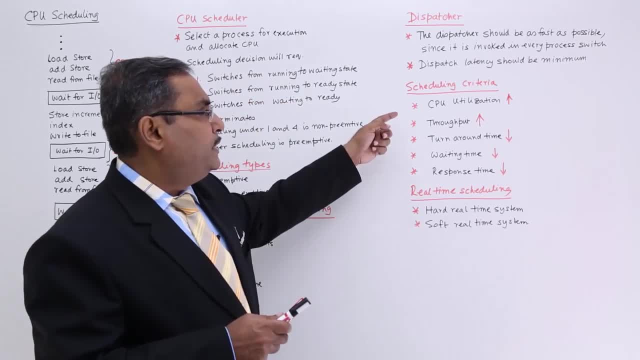 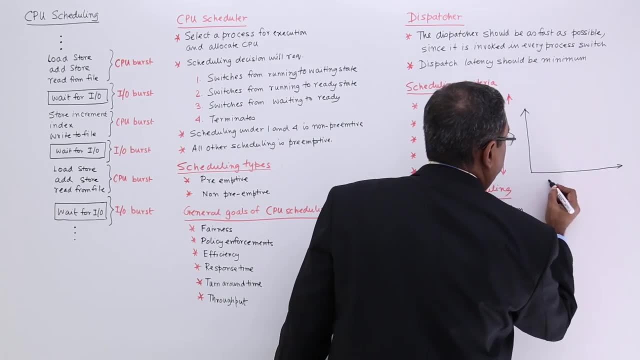 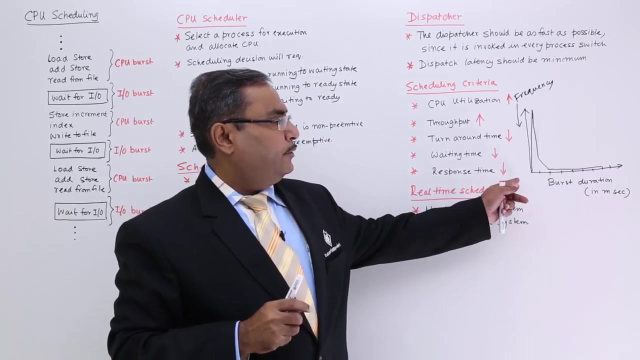 stay idle. so we cannot expect more than 90 percent of this cpu utilization for your. for your better understanding, i can draw one graph here. so here we are writing bars time now. if you consider this particular graph, you can see that along the x-axis i have plotted: 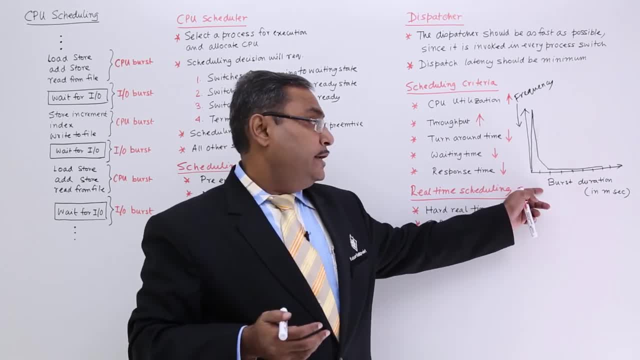 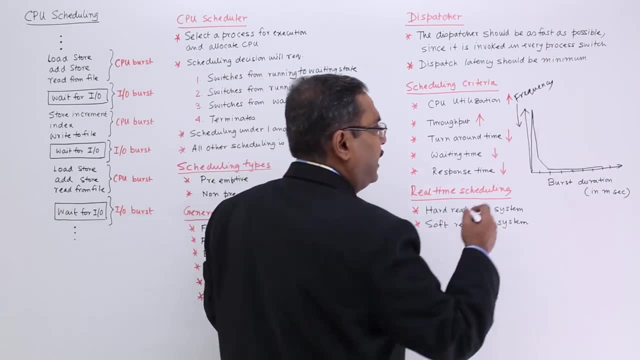 burst duration, that is a cpu burst duration in millisecond and along the y-axis i have plotted the frequency. i'm going to plot the duration of the cpu and i'm going to plot the frequency of the cpu duration. am finding that in this particular graph, the burst duration, burst duration means the cpu. has been required here at a stretch. the cpu has been required here at a stretch. cpu burst duration. you can find that the burst duration cpu burst duration minimum is having the frequency highest. that means at a stretch the cpu required by the number of times will be higher than. 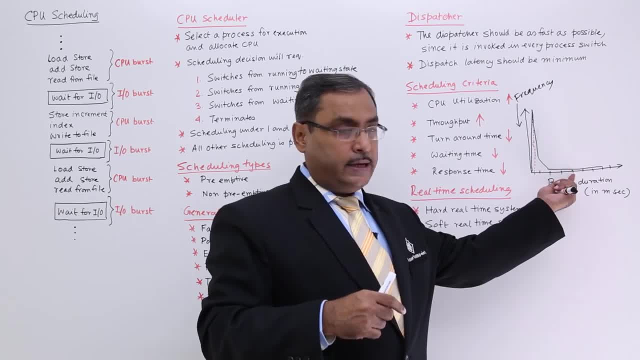 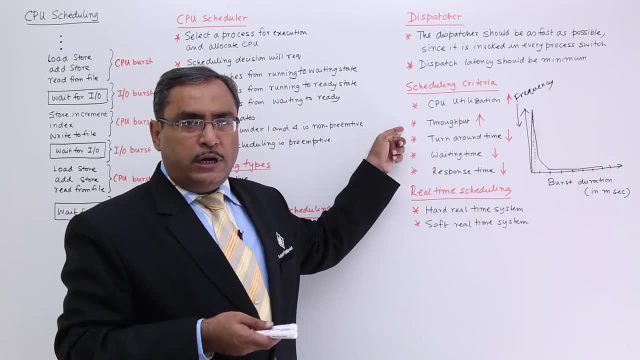 the burst duration. here the burst duration is highest or higher, but it is having the frequency very low. so that is why cpu scheduling is required. ok, so next one is the throughput. i told you earlier that the number of processes completed per unit time will be known as the 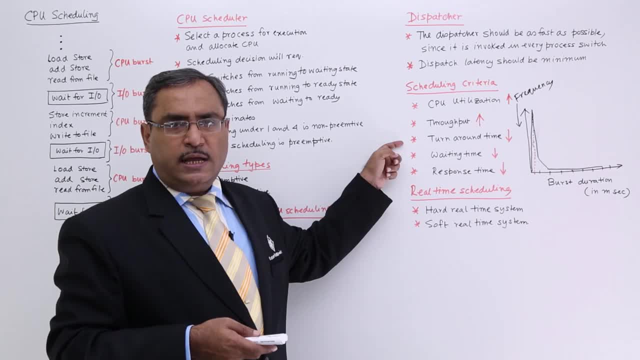 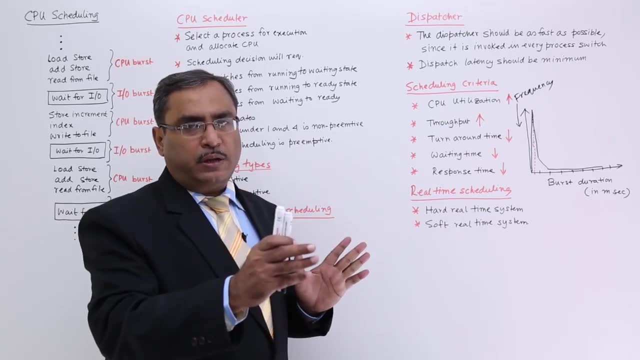 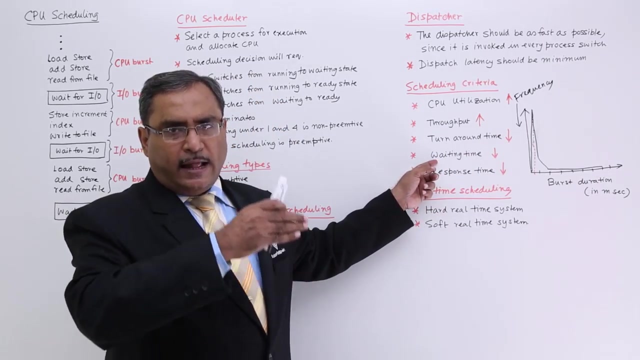 throughput: turn around time, the submission of a process and the first response. sorry, this is the response time. turn around time means the submission of the process and the completion of the process. the time gap will be known as the turn around time- waiting time- the submission of the process and the termination of the process in this particular time period. 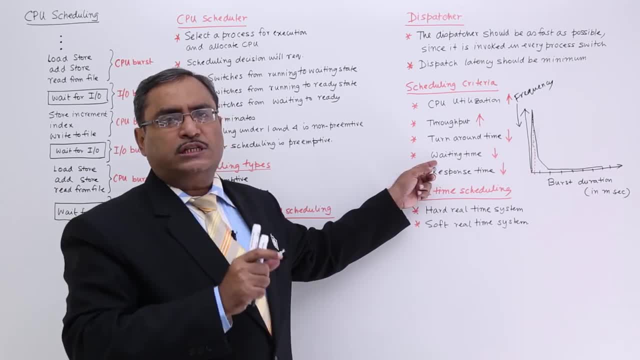 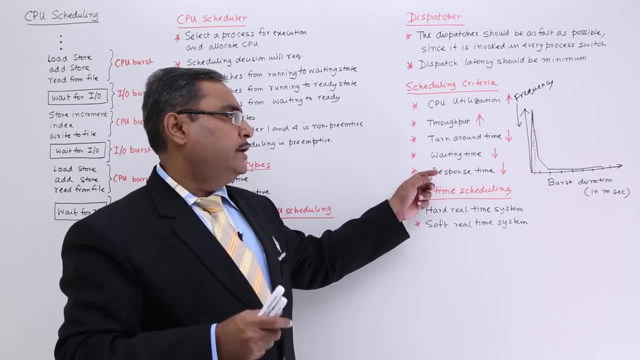 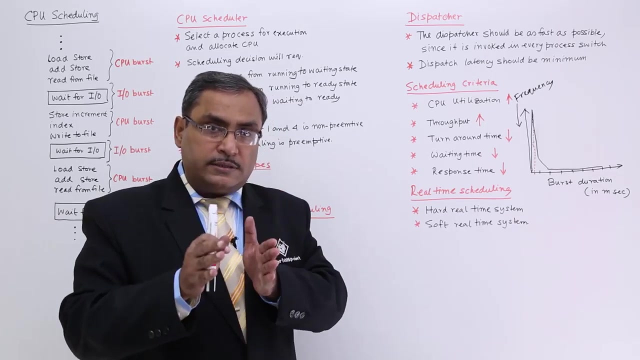 for different discrete time interval, the process may have to wait. and if you go on adding, if you go on accumulating all this waiting time, the time does obtained is known as the waiting time. so that means in the process lifespan in different discrete intervals, the process may have to wait. and if you go on adding all this waiting time, that time does obtain there. 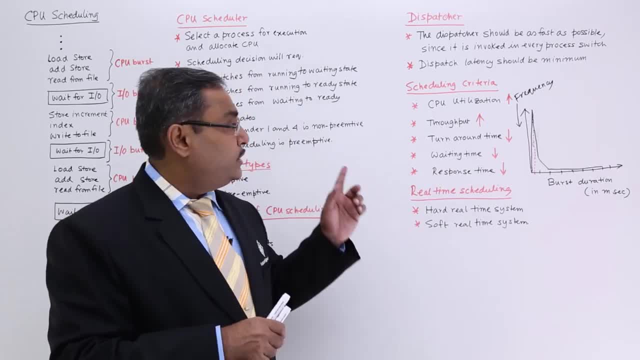 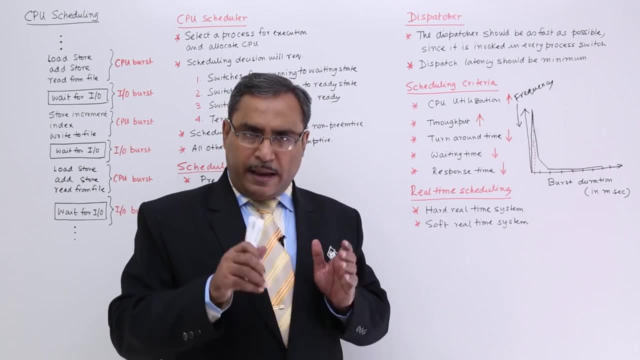 will be known as a waiting time. The last one is a response time, which I discussed earlier. Response time means the submission of the process and the first response obtained from the system. the time duration required is known as a response time. Always, we will try. 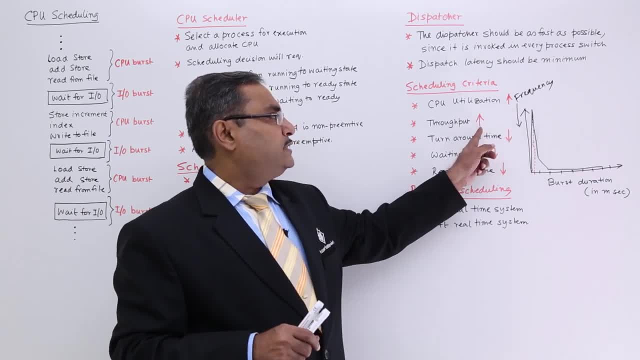 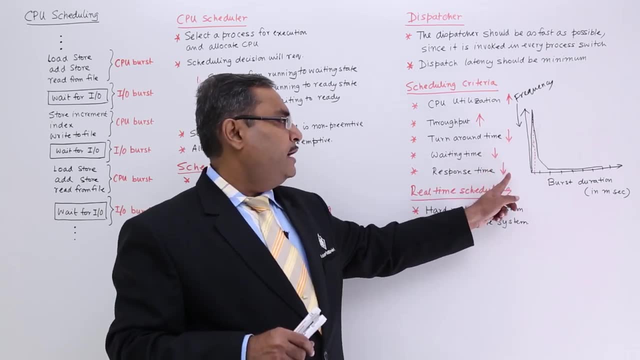 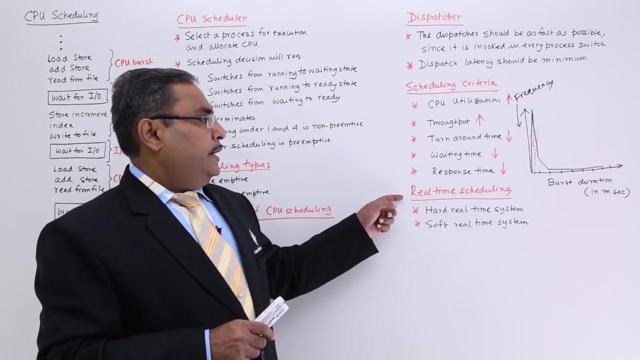 to maximize the CPU utilization, maximize the throughput, minimize the turnaround time, minimize the waiting time and the response time. So if you can do that, one that is going towards the betterment of the system, In case of real-time scheduling we can have. 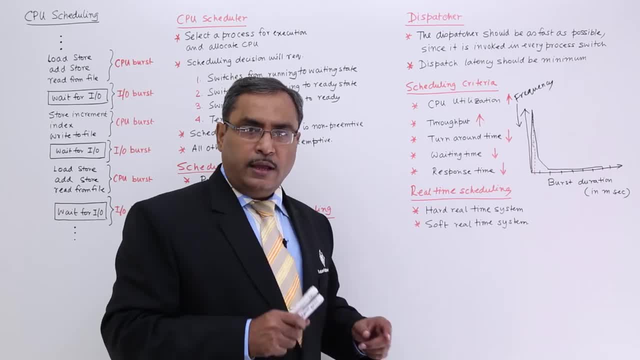 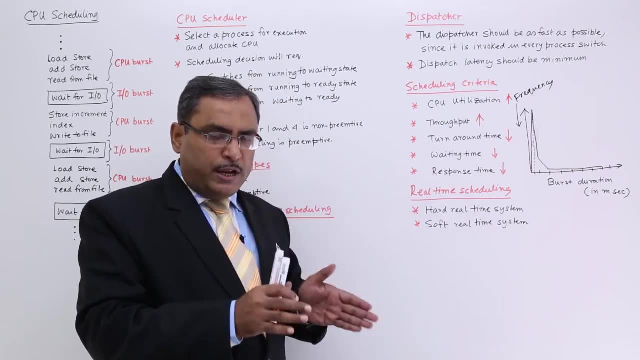 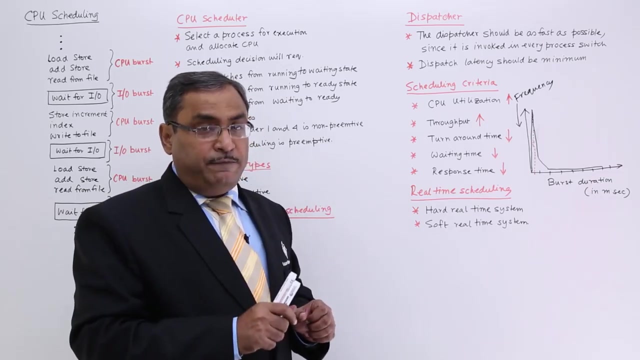 two criteria or two types. One is a hard real-time system. that means here the hard real-time system means and soft real-time system means here, in case of process completion, where having a predefined time within the frame the process has to be completed And if it is hard, bound. 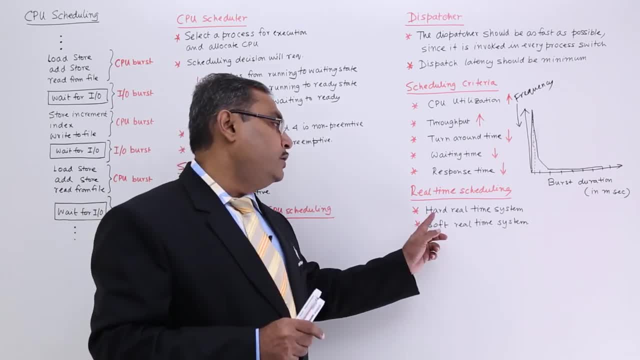 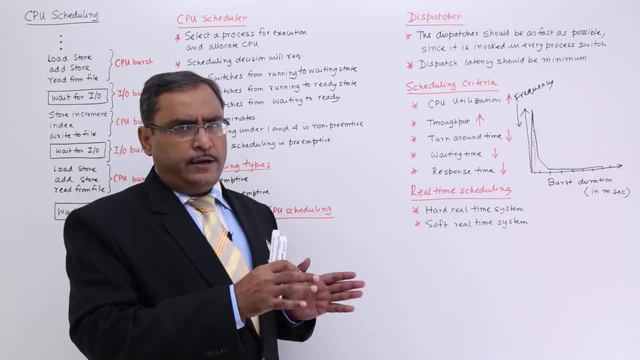 it is must to be completed within that period of time, then it is called hard real-time system. Otherwise it is not possible to complete the process within that period of time. So otherwise, in case of soft real-time system, this constraint is little bit fade, This constraint. 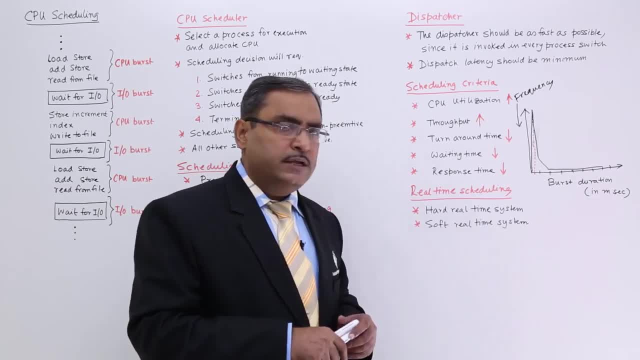 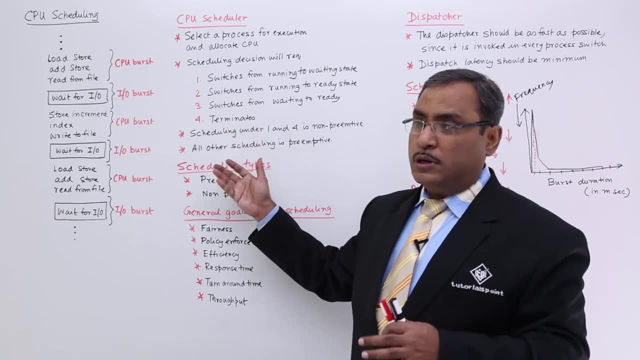 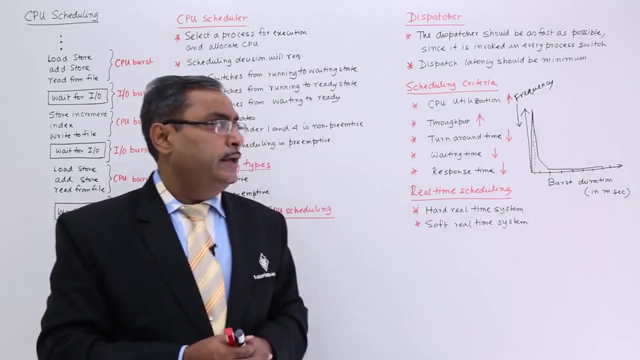 is not so hard. It is so known as soft real-time system. So, in this way, why the CPU scheduling is required and what are the CPU when the CPU scheduler will work and what are the scheduling types and what are the goals for which we should learn this particular CPU scheduling? 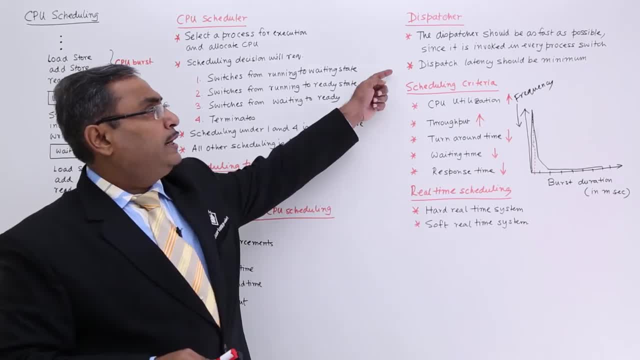 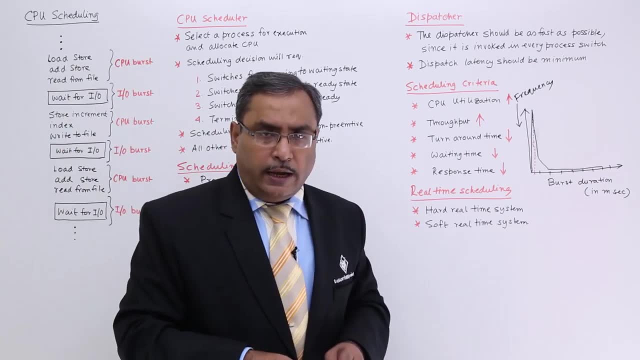 and implement this particular CPU scheduling in our systems and what is a dispatcher scheduling data? I have discussed each and everything in this particular session. I think we have got the logic why the CPU scheduling is required and what is about. I think you can answer. 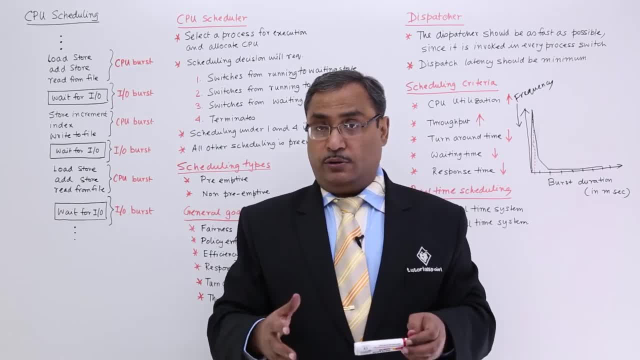 questions. if the questions comes on this particular CPU scheduling- and it is bound to come- I can tell you that one Thanks for watching this video.